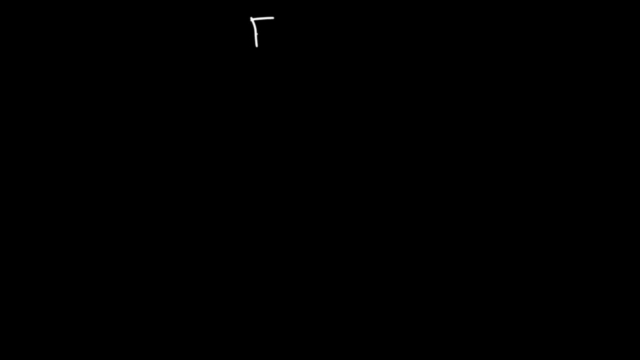 Now let's talk about even and odd functions. Let's go over the even functions first. Cosine is an even function. Cosine of negative x is equal to cosine of x, And a reciprocal of cosine which is secant is also an even function. Secant of negative x is equal to. 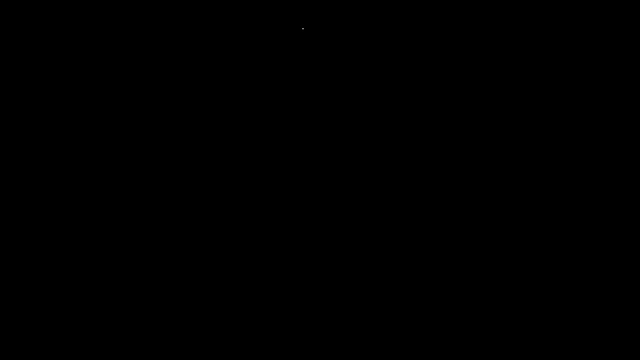 secant x. So those are the even functions. The other four are odd trigonometric functions. So, for example, sine of negative x is negative sine x- Notice that the sine changes. And cosecant, which is a reciprocal of sine, is also an odd function: Cosecant negative x. 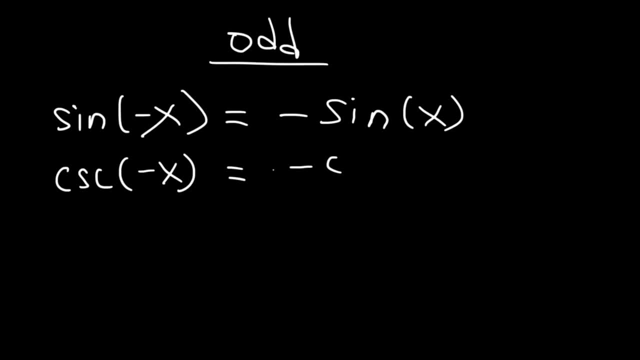 is negative cosecant. I was about to write cosine: negative cosecant positive x. So the tangent is also an odd function. Tan negative x is negative tangent x And also cotangent of negative x is negative cotangent of x. So those are the even and odd trigonometric. 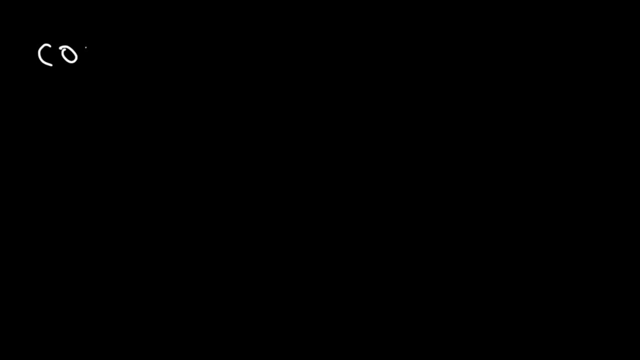 functions. Now how do we apply this information? So let's say, if we want to find the value of cosine of negative 45 degrees, Well, we know that cosine of negative 45 degrees is negative. x is simply positive cosine of positive x. So therefore, cosine negative 45 is equivalent. 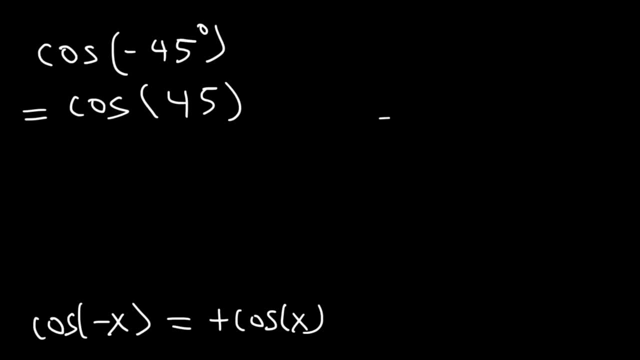 to just cosine of 45. Now, using the unicircle, we know that 45 corresponds to the point square root 2 over 2 comma, square root 2 over 2.. So cosine 45 is root 2 over 2. And we know. 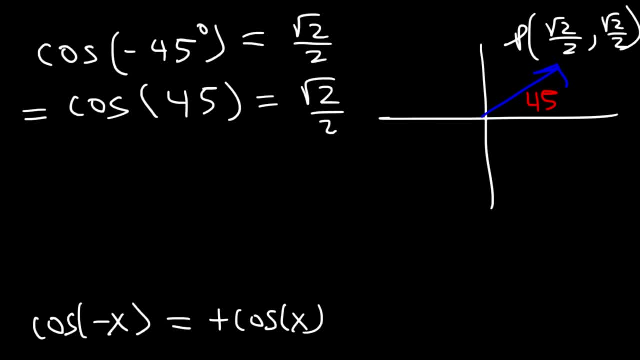 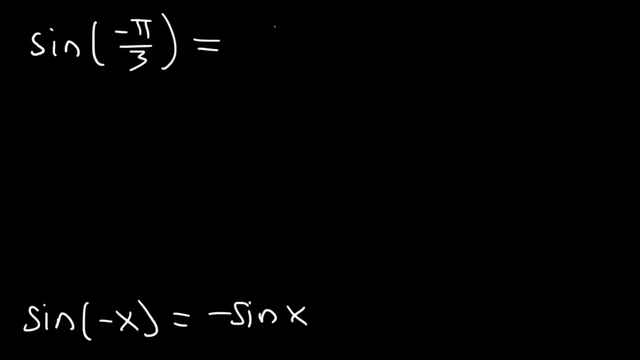 that cosine of negative 45 is the same thing root 2 over 2.. So these are the same. Now, what about sine of negative pi over 3? We know that sine of negative x is negative sine x. So therefore, sine of negative pi over 3 is negative sine pi over 3.. 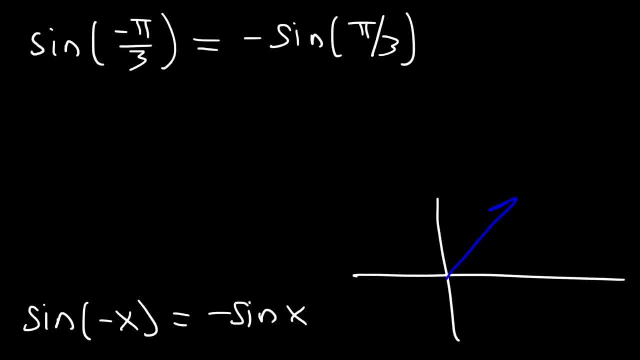 So at an angle of pi over 3, this corresponds to the point of the unicircle which is one half root 3 over 2.. And sine is associated with the y value. So sine of pi over 3 is positive root 3 over 2.. But with a negative sine in front. sine negative pi over 3 is: 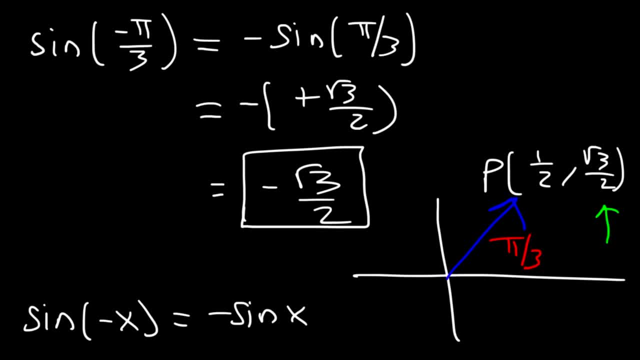 going to be negative root 3 over 2. And negative pi over 3, it's basically going to be negative 3 over 3.. So sine of pi over 3 is going to be negative, sine pi over 2. So this one is negative. So sine of pi over 3 and sine of pi over 3 is negative sine pi. 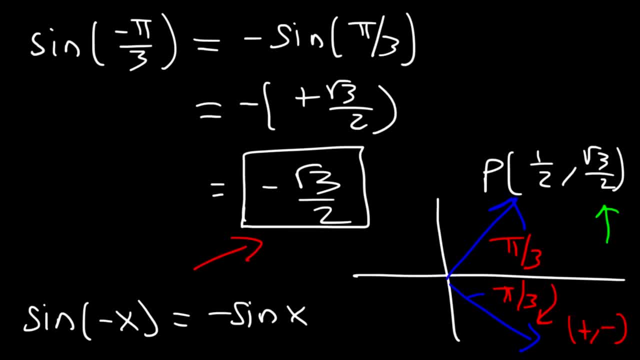 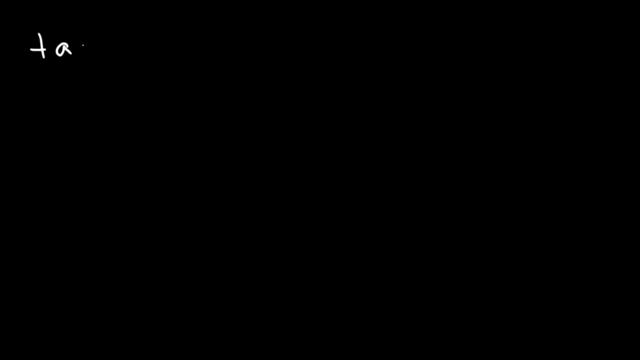 over 3.. So in the fourth quadrant we have a negative sine, And so thus this is an agreement with the answer that we have negative root 3 over 2.. Now what about tangent of negative 3 pi over 4? Let's try that one. 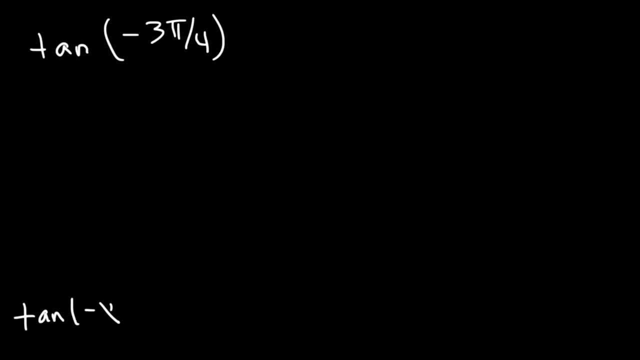 So tangent of negative pi over 4, we have an angle of that wood square root, x, so it's negative. X is an odd function, so this is negative tangent of X. so therefore this is going to be negative tangent of 3, pi over 4. now, at pi over 4 we have the 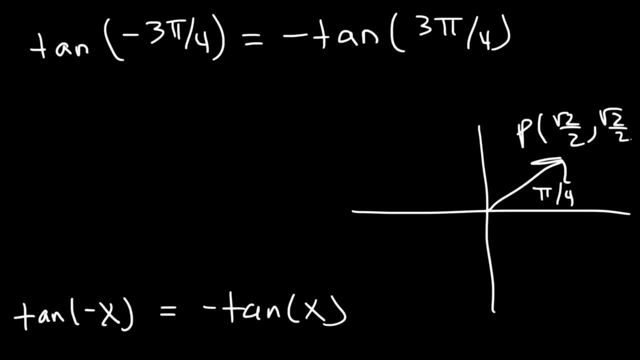 point: square root 2 over 2. comma: square root 2 over 2. now at 3 pi over 4, which is in quadrant 2, we have a similar point, but only X is negative, Y is positive. so, if you recall, tangent is going to be Y divided by X, in this case at 3 pi over 4. 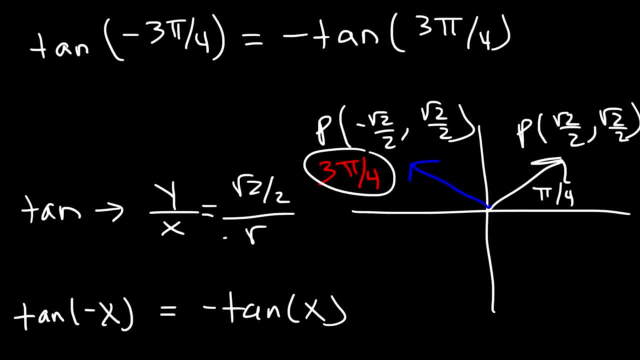 we have root 2 over 2 divided by negative root 2 over 2, so the square root 2s will cancel, the 2s will cancel, and so we're left with root 2 over 2 is just 1, but this one is negative, so overall it's. 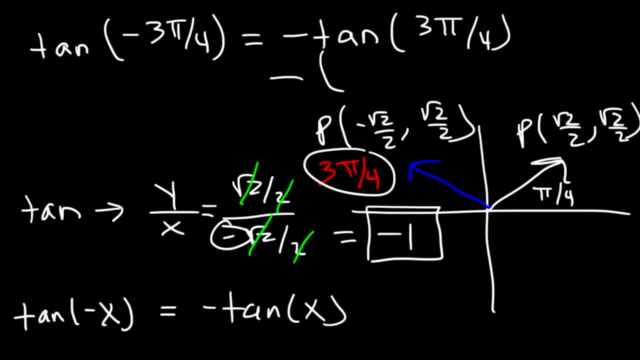 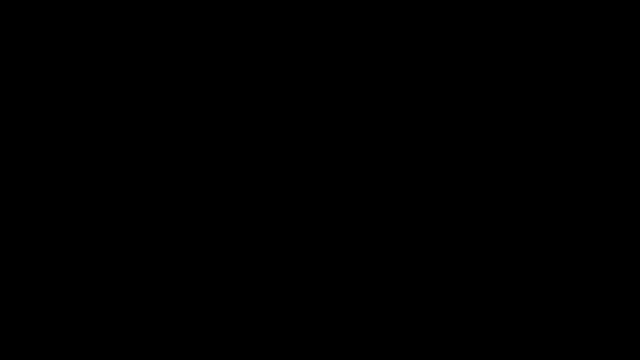 going to be negative 1. so tangent 3 pi over 4 is negative 1. but negative times negative is going to equal a positive value. so tangent of negative 2 pi over 4 is positive 1. now let's make sense of it. so here's 3 pi over 4. 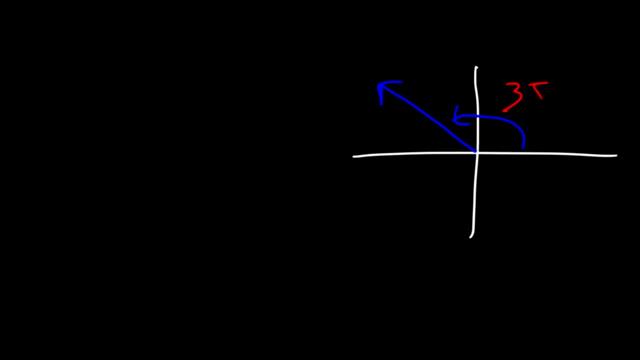 it's in quadrant 2, and in quadrant 2 we know that X is positive, Y is negative. so because tangent is Y over X, when you take a negative value and divided by a positive value, you get a negative result. that's why tangent 3 pi over 4 was a. 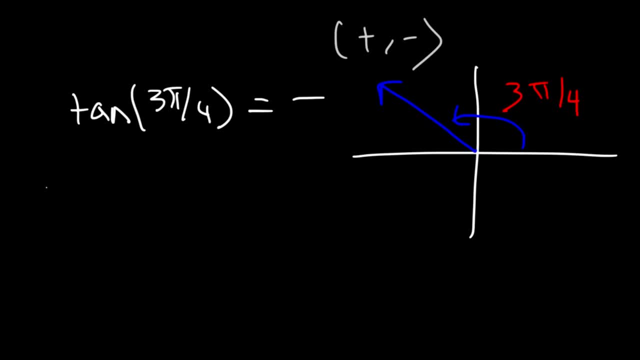 negative answer. now what about tangent of negative 3 pi over 4? so to get negative 3 pi over 4, we need to go in the other direction, which is here, and notice that negative 3 pi over 4 is in quadrant 3 and in quadrant 3, X and Y. 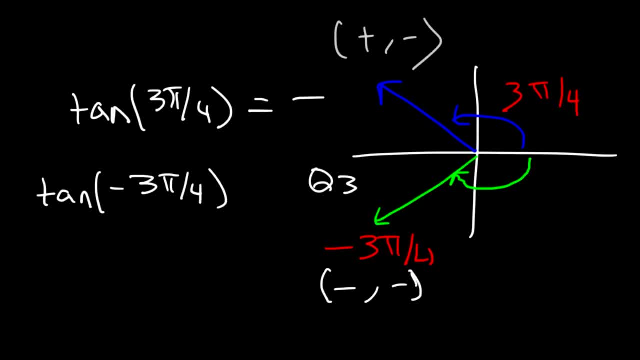 are both negative. so tangent, which is Y over X, if you take a negative number and divided by a negative number, you're going to get a positive value, and so that's why tangent 3 pi over 4 was negative 1. but tangent negative 3 pi over 4 was positive 1, which makes 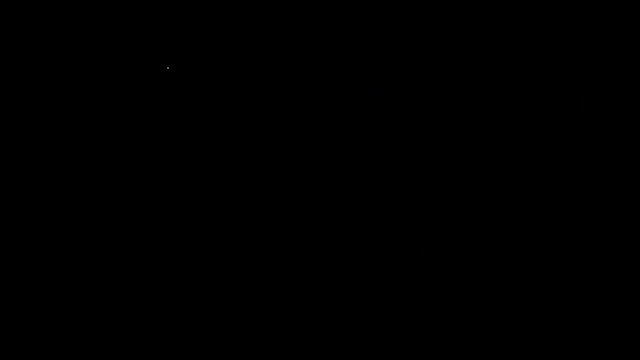 an odd function. now try this one: cosecant of negative 5 pi over 6. now, cosecant is reciprocal of sine, so therefore cosecant is going to be an odd function. so this is equal to negative cosecant of positive 5 pi over 6. now, 5 pi over 6 is: 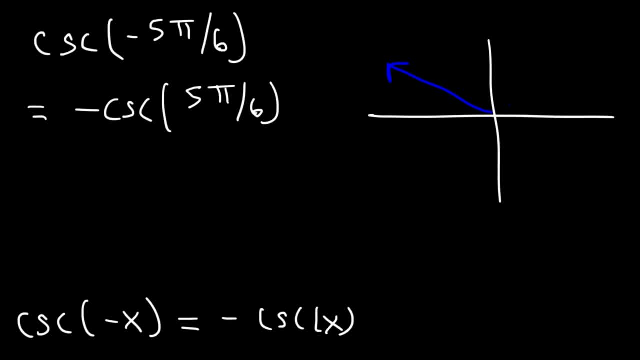 pi divided by 6, and we know the point for pi over 6, it's root 3 over 2, comma 1 half. so 5 pi over 6, which is in quadrant 2. we only have to change the x coordinate. now cosecant is 1 over sine. 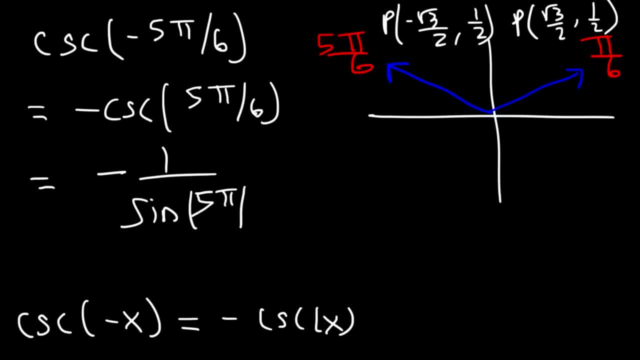 and sine 5 pi over 6 corresponds to the y-value, which is 1 half. so sine 5 pi over 6 is positive 1 half and 1 divided by 1 half is 2, but overall it's negative 2. so therefore cosecant negative 5 pi over 6 is negative 2. negative 5 pi over 6 is in. 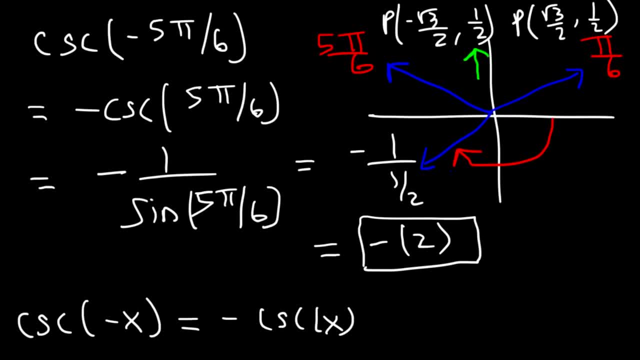 quadrant 3 and in quadrant 3 the y-value is negative, and so that's why cosecant negative 5 pi over 6 is going to be a negative answer overall, because if you actually plot this, this will take it to quadrant 3, and in quadrant 3 y is 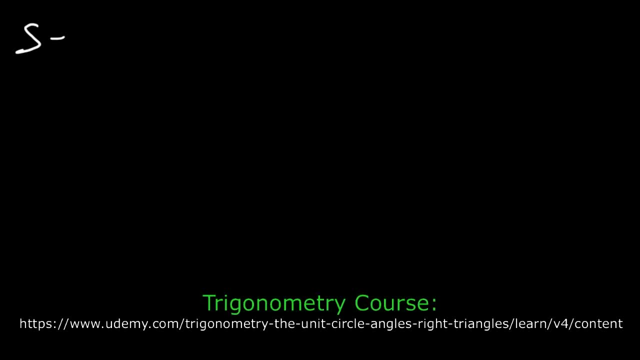 negative. let's try a secant of negative 11 pi over 6. so feel free to pause the video and work on that example now. secant is an even function because it's a reciprocal of cosine, which is also even. so secant negative x is the same as secant x. so basically we're 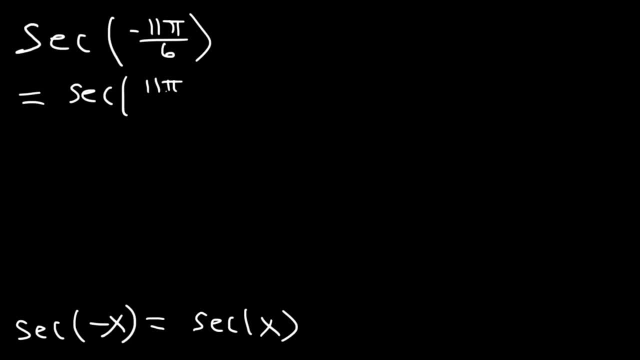 looking for a secant of positive 11 pi over 6. 11 pi over 6 is in quadrant 4 and pi over 6 is in quadrant 1. in quadrants 1 and 4, cosine is positive and secant which is 1 over cosine is also positive. therefore, 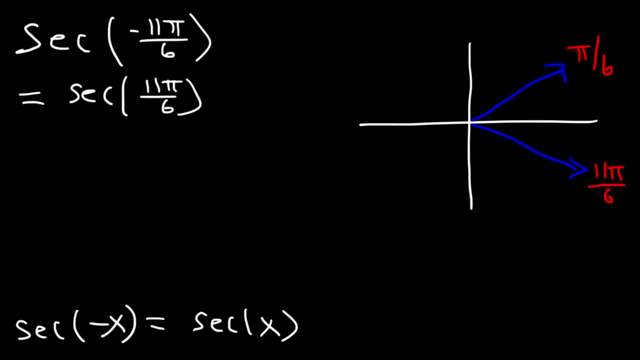 our final answer should be positive now at pi over 6, which is 30 degrees. we have this point. so 11 pi over 6. only the y-value changes. x is negative in quadrants 2 and 3, but x is positive in 1 and 4 and y is negative in quadrant 4, right? 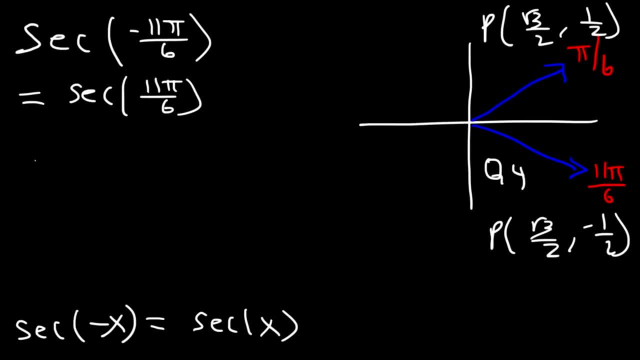 now this is in quadrant 4. now, using the reciprocal identity, we know that secant is 1 over cosine and cosine corresponds to the x value. so at 11 pi over 6, cosine is root 3 divided by 2, and 1 divided by root 3 over 2 is going to be: